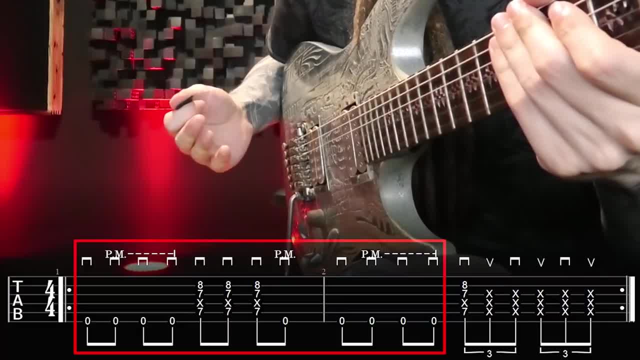 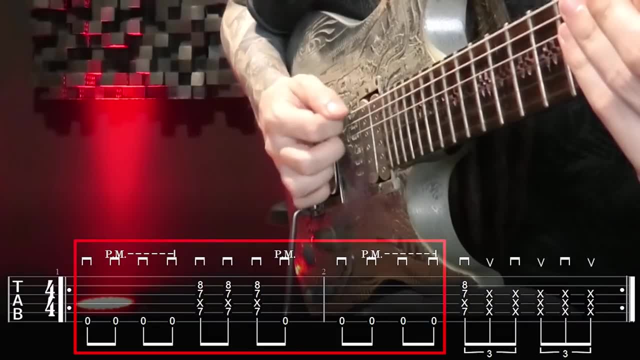 and eighth note triplets played with alternate picking. For the first group of notes- the eighth notes- with downstrokes, your picking hand will be resting on the bridge so that you can switch between open notes and palm muting, and for the second, faster group, you will slightly lift your hand and switch to your strumming. 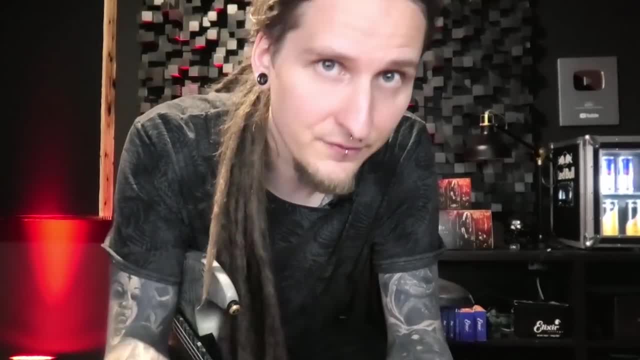 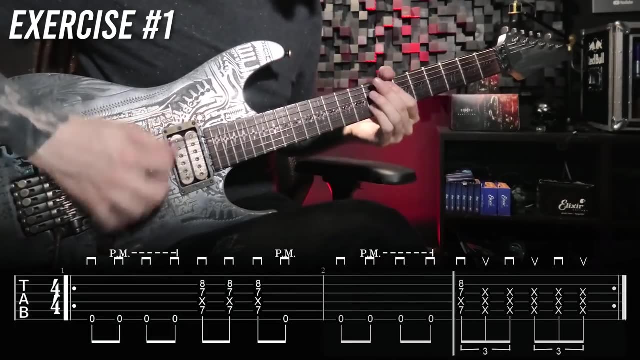 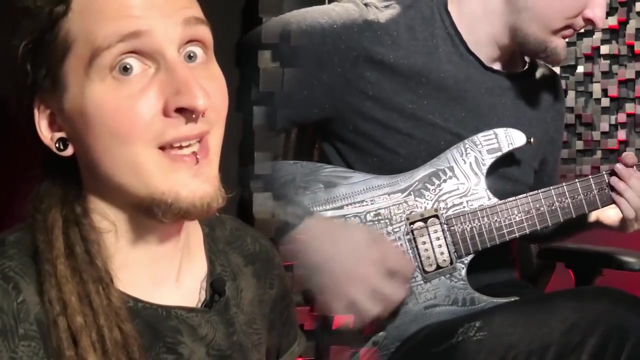 technique so that you can easily play the dead notes in between. Here's how this first exercise looks like. It's really difficult not to rush as soon as you play those eighth note triplets and then to drag, And of course it's also tricky to switch between the picking motion and the strumming. 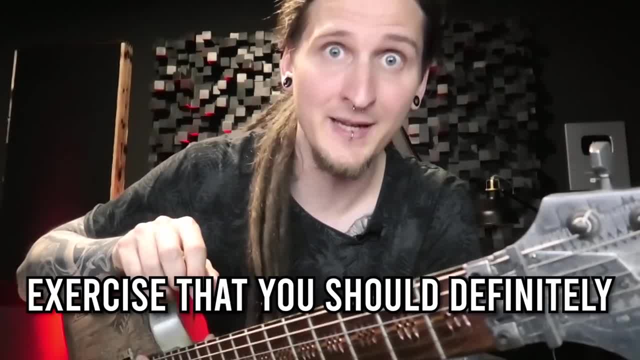 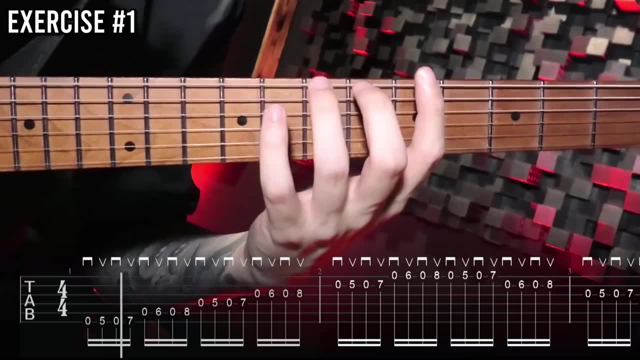 motion- quite a lot to keep in mind. so this is an awesome timing and rhythm exercise that you should definitely work on each day. Make sure to download all the really helpful practice files I made especially for you on Patreon. I always make downloadable exercise video, playalongs, PDF tabs, backing tracks, guitar. 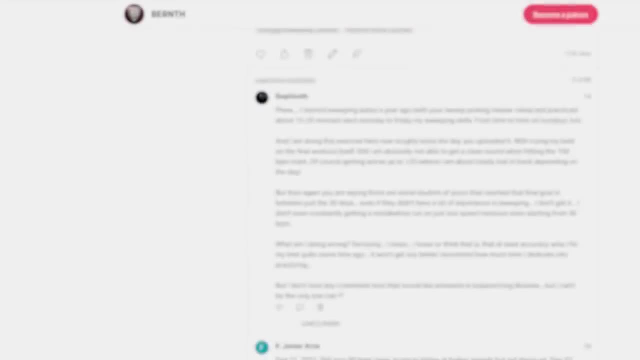 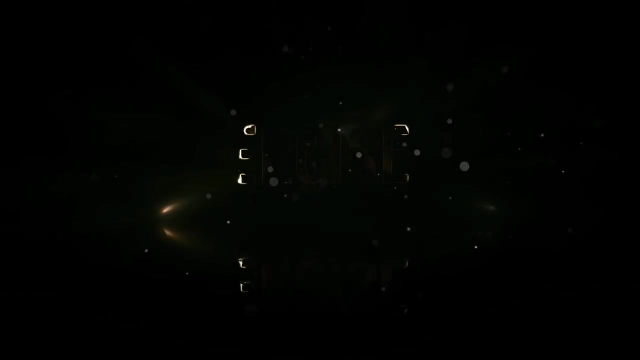 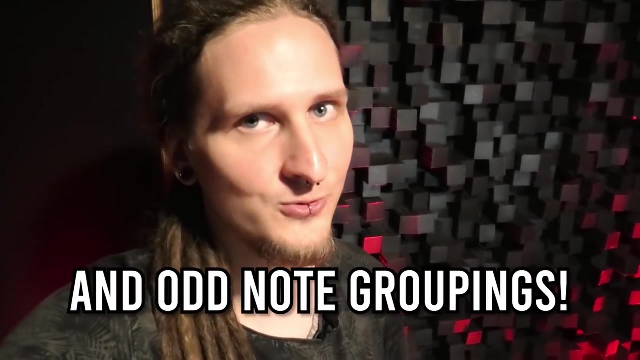 pro files and even full online courses for our awesome community of over 4000 dedicated players over there. So join us today. the link is in the description and in the first comment below. Alright, the second exercise is all about rhythmic displacement and odd note groupings. 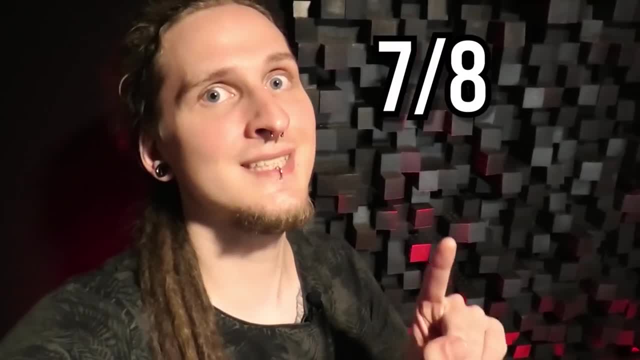 With this one, I'd like to show you that you don't necessarily need odd meters like 7, 8 or 5, 4 to create complex and intriguing riffs. you can also do it in good old 4, 4!. 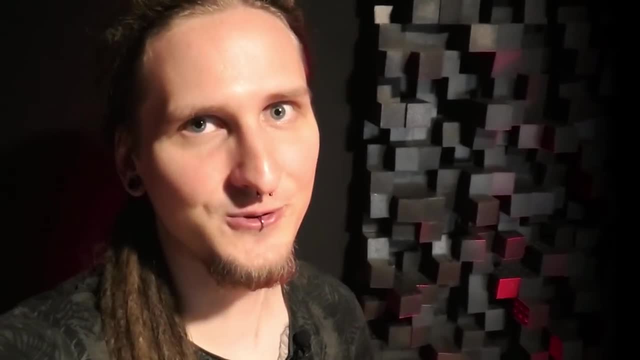 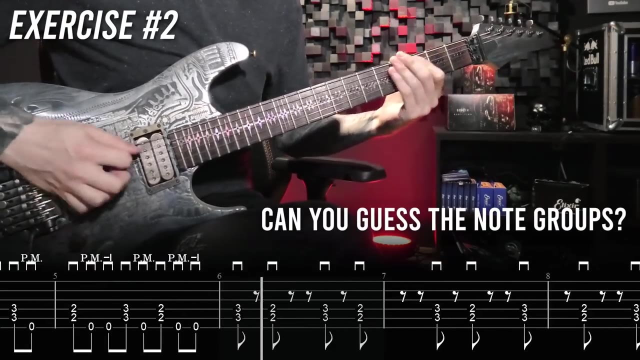 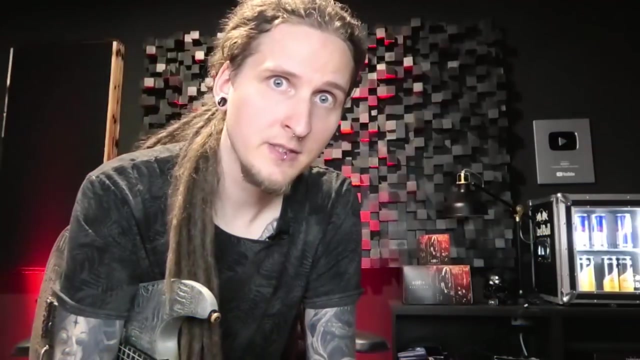 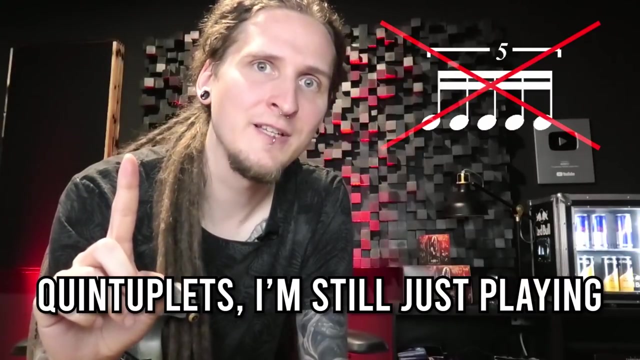 And here's an awesome example exercise that features this system that I want to show you. With this one I was playing groups of 5 8th notes in a 4, 4 time signature. please remember those are not quintuplets. I'm still just playing regular old 8th notes here, but by 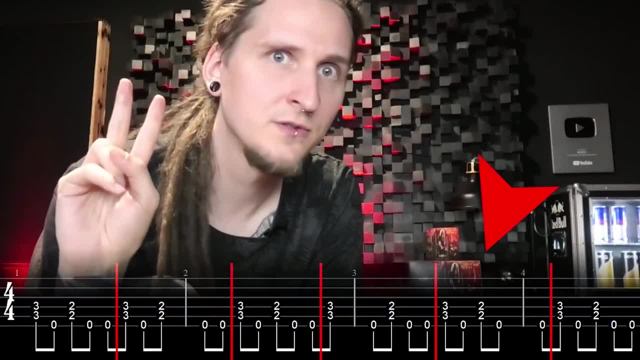 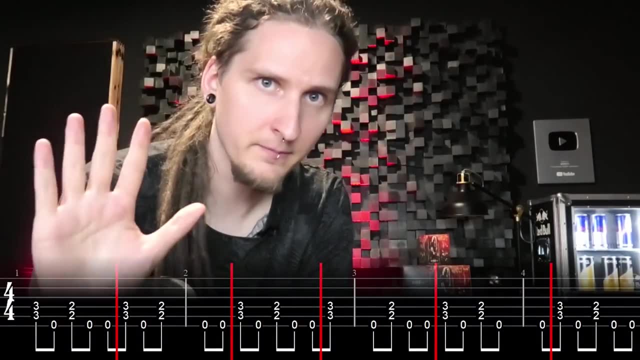 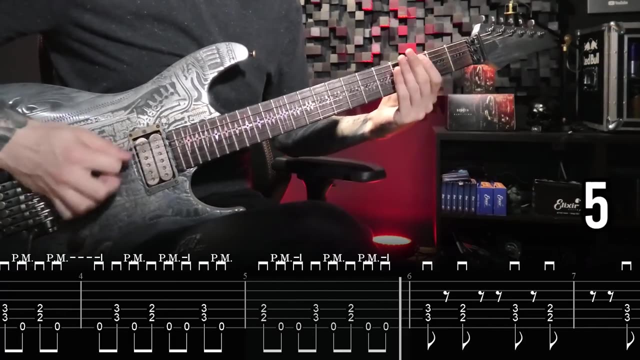 rhythmically dividing them into groups of 5 instead of your usual groups of 2 or 4, the accents created by that keep drifting away from the beat until the pattern finally repeats after 5 measures. And to make all this even crazier, I didn't just repeat the riff after 5 measures, I only 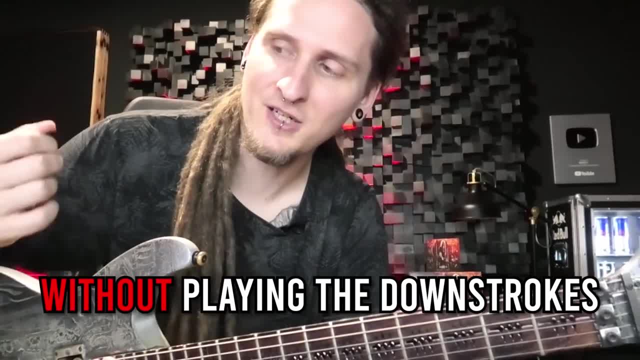 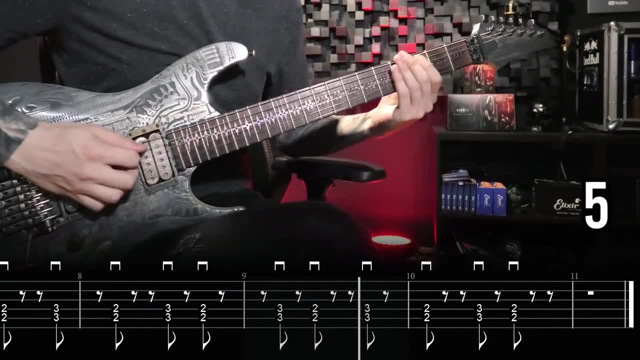 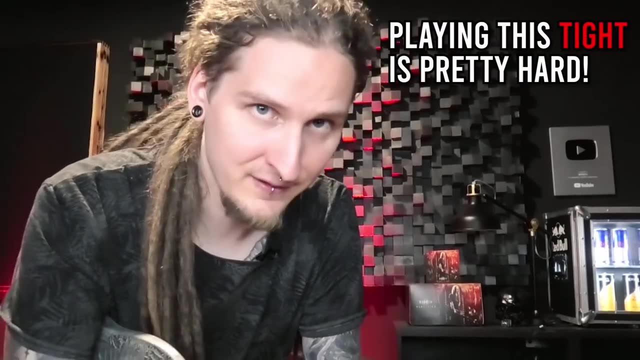 played the accents on the A and D strings without playing the downstrokes on the low open E string in between. So this sounds really cool and kind of crazy played against that straight rock beat and it's actually quite difficult to really nail those odd accents in time. 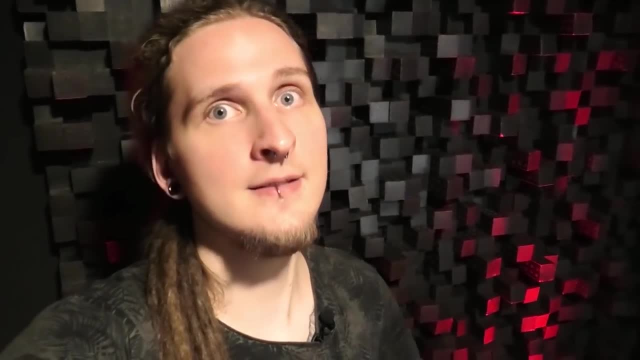 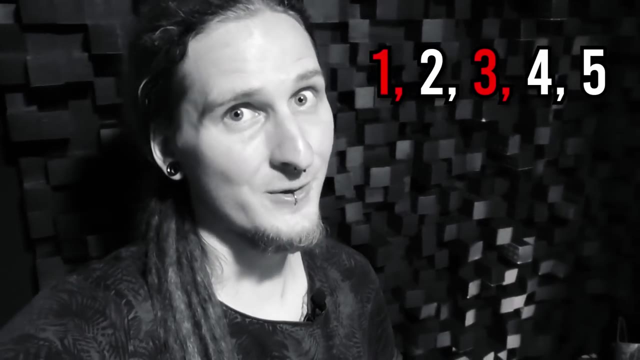 My personal trick concerning that is just counting the 8th notes in my head In groups of 5, and I'm just playing the 1st and the 3rd note, but since the tempo is kind of fast I can't just count in numbers anymore. 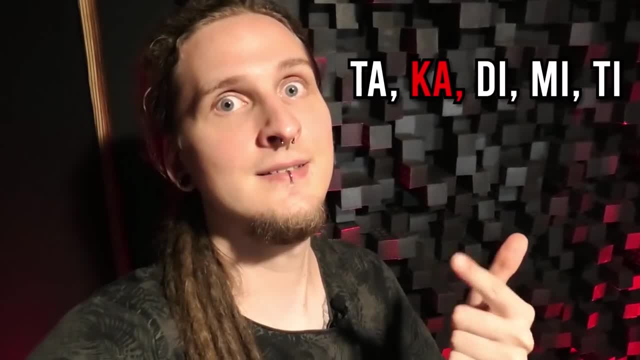 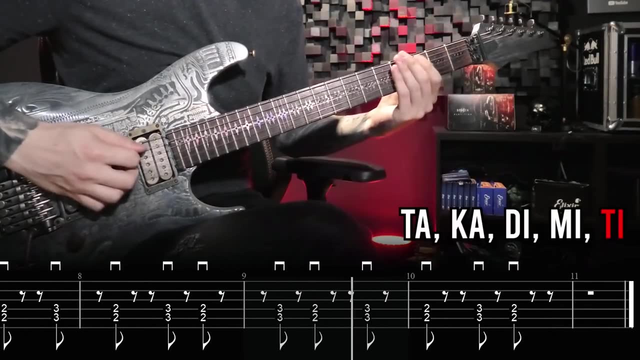 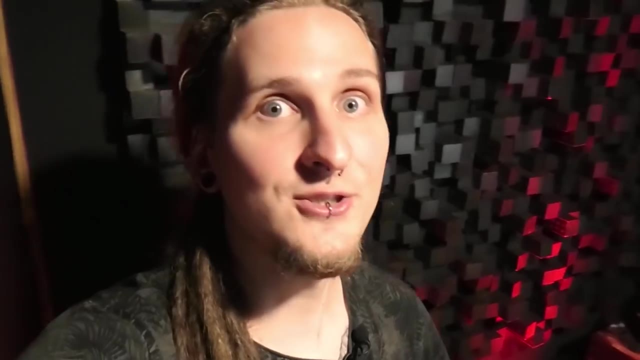 That's when I like to use Connor Cole inspired phrases like ta-ka-di-mi-ti for groups of 5!. Connor Cole is the art of performing percussion syllables vocally in Indian music, and you should really look into this if you're searching for a better system of counting than 1234512345!. 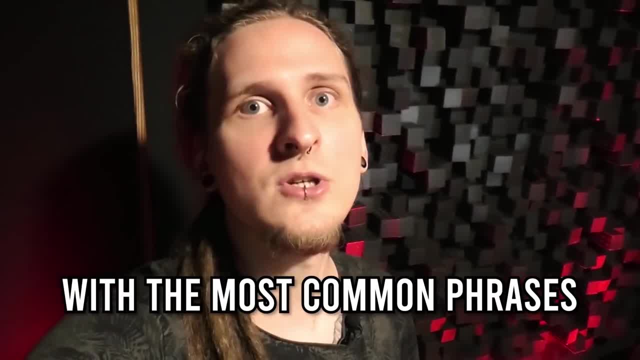 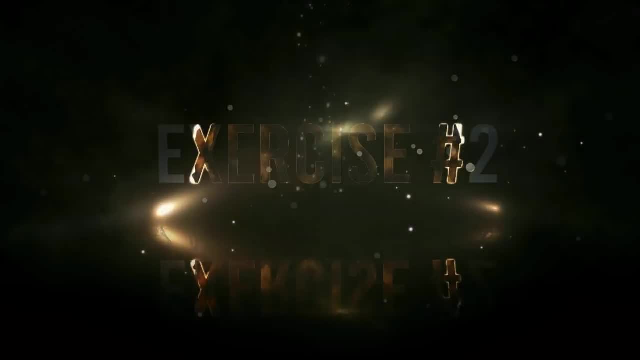 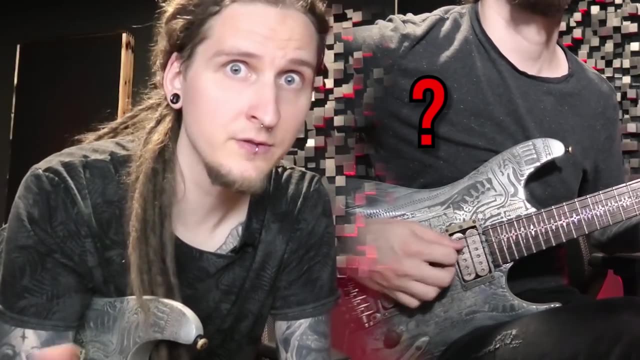 Of course, I made sure to create a helpful sheet for all patrons with the most common phrases. that way, you can learn to start counting like this with groups of 2,, 3,, 4 and 5!. So in case this second exercise is a bit too rhythmically challenging and confusing for you, 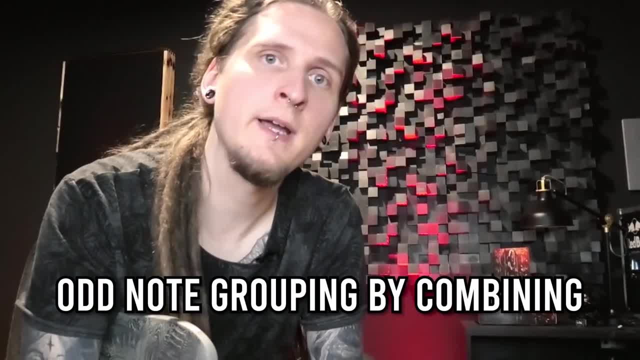 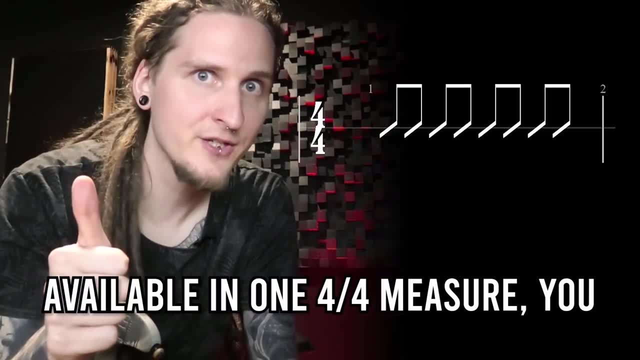 at the moment you can also start exploring odd note grouping by combining groups of 2 or 3 8th notes in just one note. Since you just have 8 8th notes available in one 4-4 measure, you end up with the following: 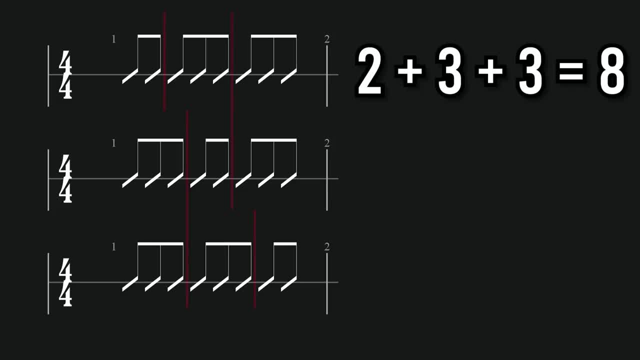 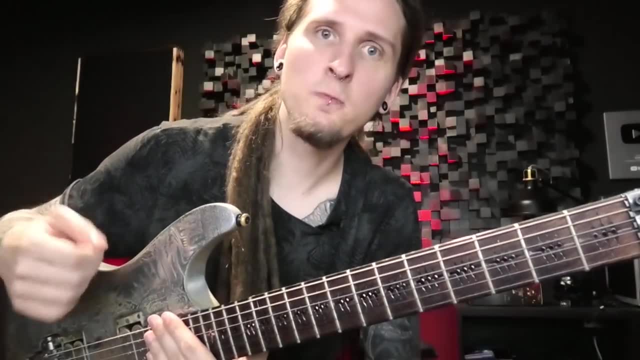 possibilities 2-3-3,, 3-2-3, and 3-3-2!. So for the next, more basic exercise, I'm just playing the low open E string and I'm accenting all first notes of every single group by playing E one octave higher on the 12th fret. 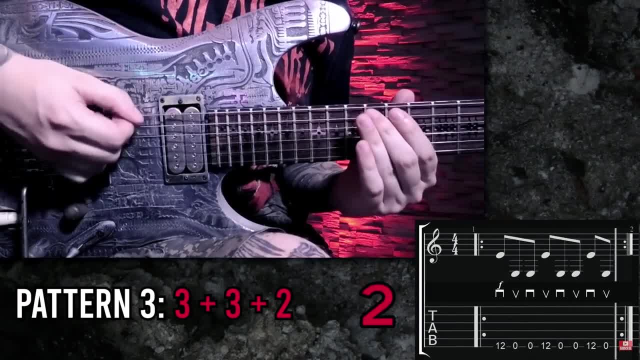 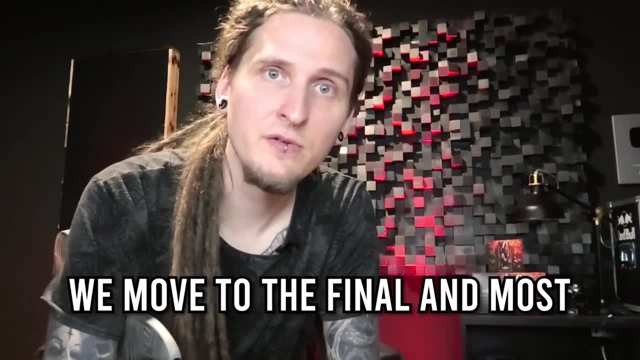 So that's a bit easier, but you still end up with tons of awesome creative possibilities for your riffs and licks. And the last thing you can do before we move to the final and most challenging exercise of this video is experimenting with just playing a repeating group of three eighth notes. 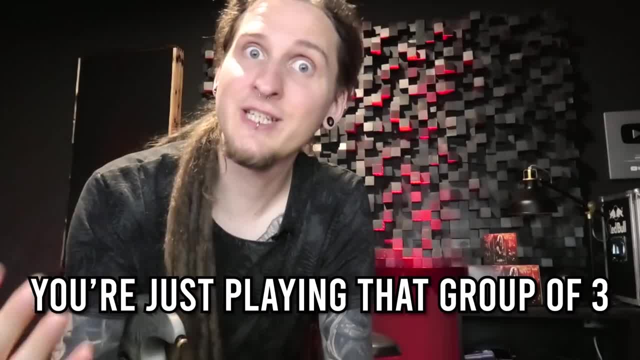 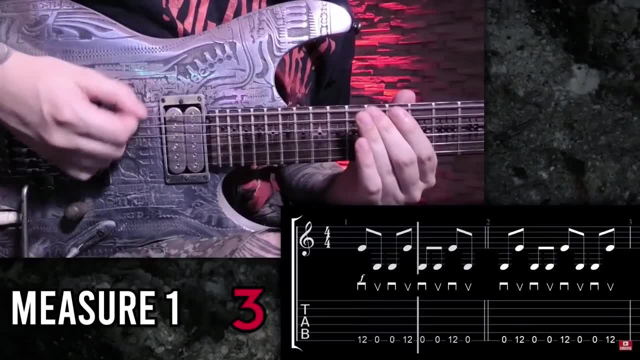 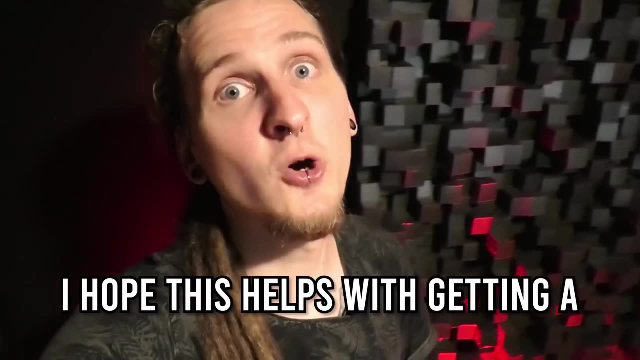 so you're not just limiting yourself to one measure anymore, you're just playing that group of three over and over again until the full pattern lands on the one again of the three measures. I hope this helps with getting a feeling for odd note grouping and rhythmic displacement at. 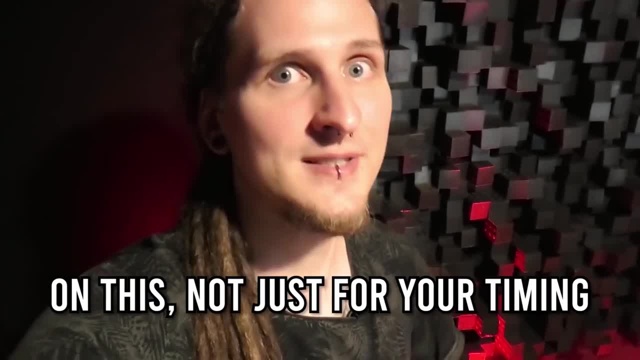 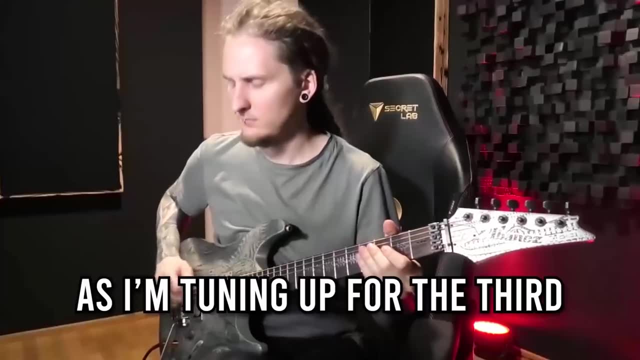 the beginning. trust me, it really pays off to work on this, not just for your timing and rhythm skills, but also to fuel your creativity when it comes to writing progressive and odd riffs and licks. As I'm tuning up for the third exercise concept I want to show you today, allow me to give you a quick 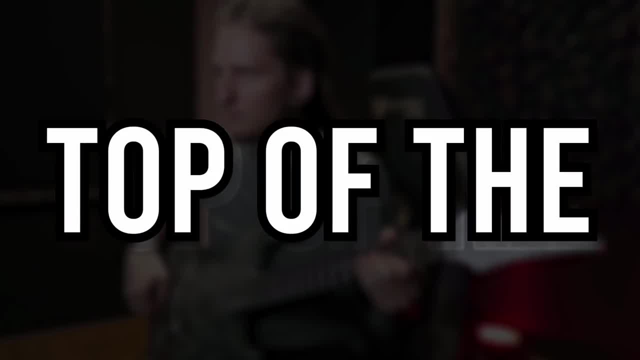 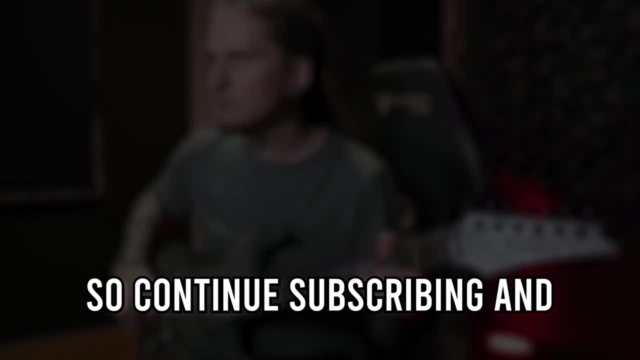 mission update. As you know, we want to take guitar to the top of the YouTube charts in Austria together. Great news: I've been to four places over the last weeks and moved to spot 86 now, so continue subscribing and spreading the message. we are really making a difference right here and I think we can actually 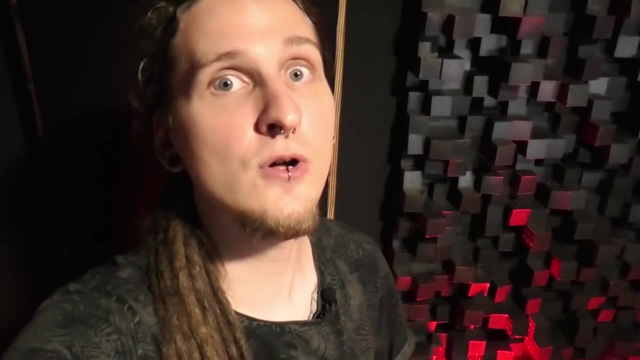 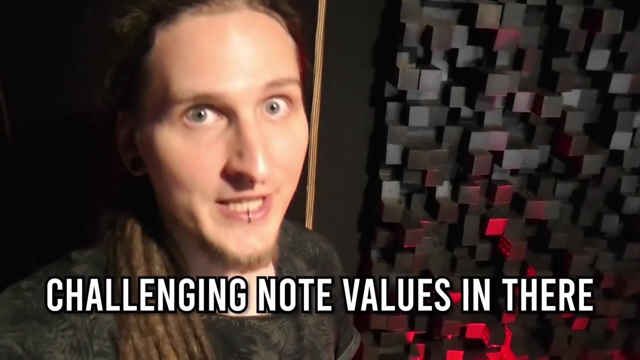 pull this off. So the third and most challenging exercise is all about involving the fretting hands on more, about switching between fast downstrokes and alternate picking, and I also added some of the most challenging note values in there: of course, the fast 16th notes, but also quarter note triplets. 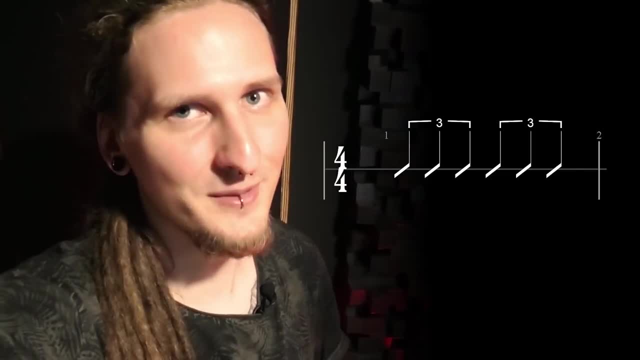 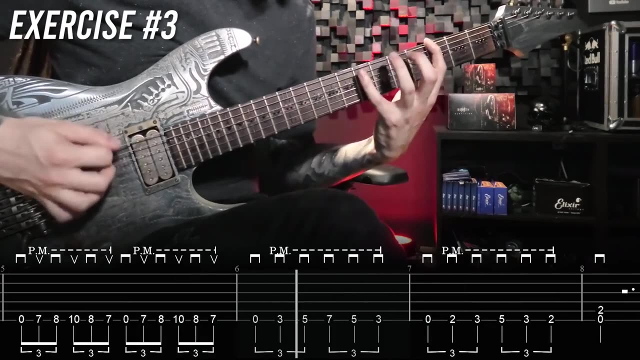 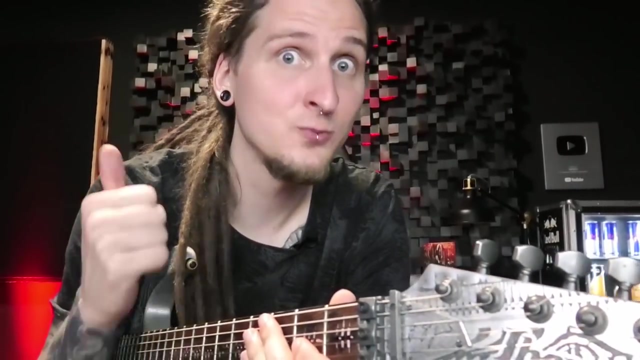 You will see they aren't exactly fast, but it's really hard to get them right here with perfect timing. So this one is quite tricky and I would suggest spending some time with exercises one and two before you tackle this third one. of course, you can also start by isolating each group before you. 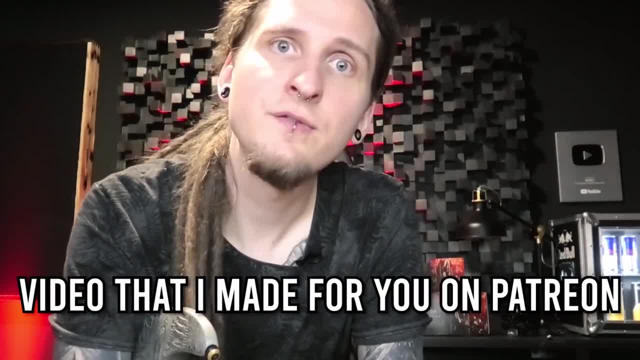 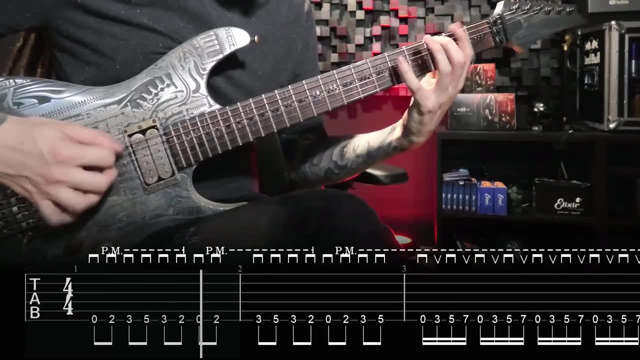 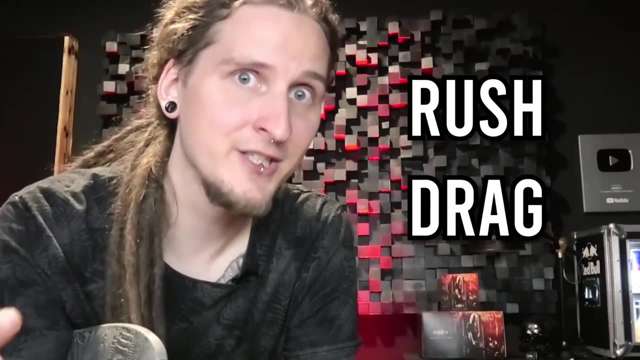 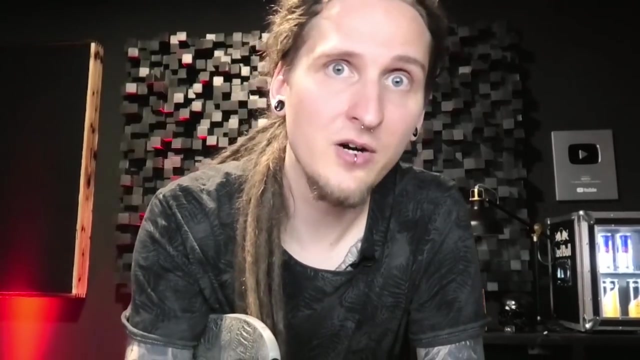 start combining them, just like with this extra practice video that I made for you on Patreon, but obviously the biggest goal is really focusing on switching between those different groups. as I said, you don't want to drag or rush after those transitions and in my personal opinion, that's the most important skill you can have as a rhythm guitar player. So to give you even more, 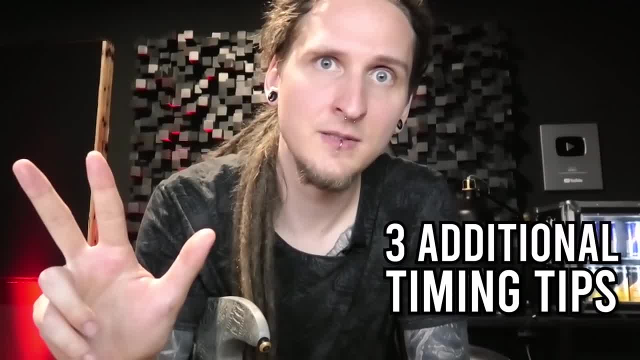 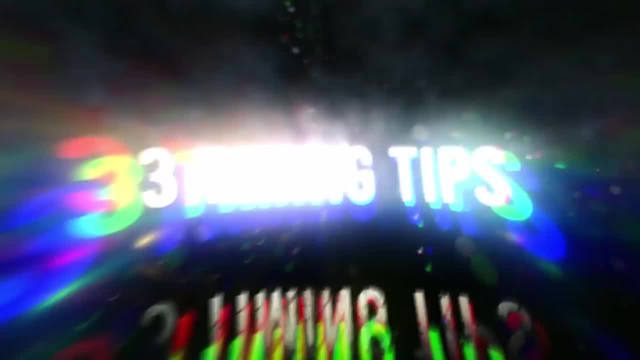 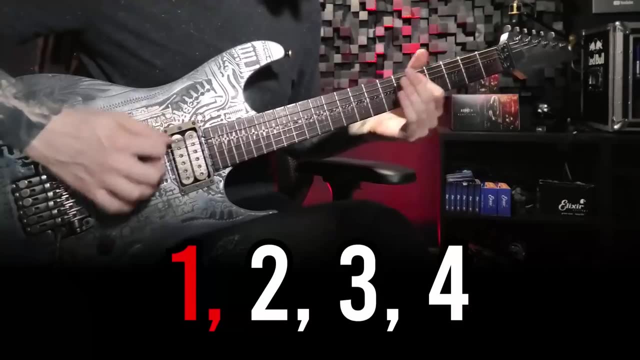 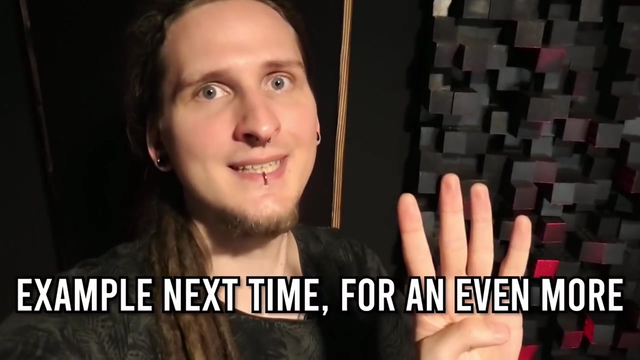 value. at the end of this video I have three additional practice tips when it comes to timing and rhythm in your practice routine. First tip: you can and should experiment with the metronome. you can start your workouts and exercises on the one try, starting on the two or four, for example. next time for an even more challenging timing twist with